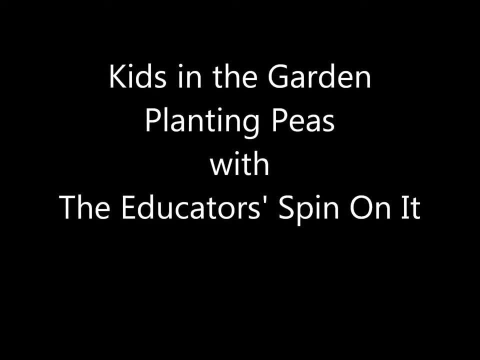 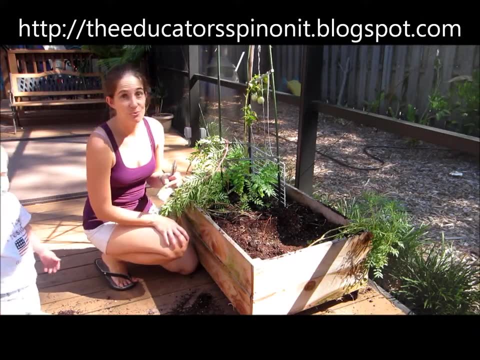 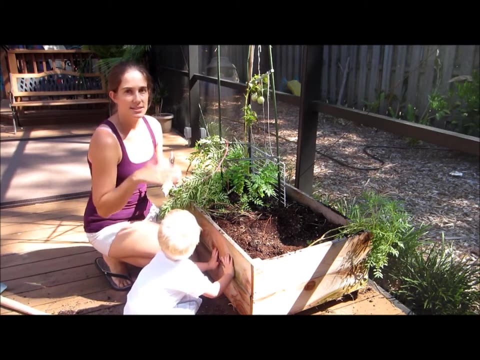 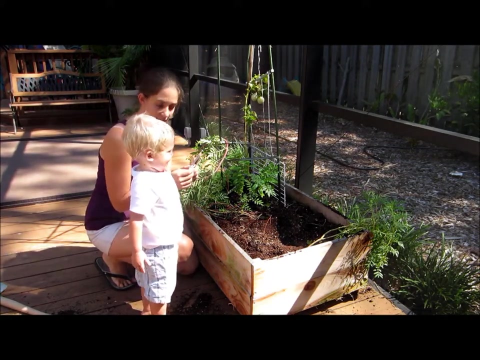 Amanda from The Educator's been on it, and today we're going to be working in the garden, and this garden is our kid garden, so I let them decide what they want and plant all of it. and Nicholas is going to be planting today and he has chosen peas, peas. he really likes to pick peas, so 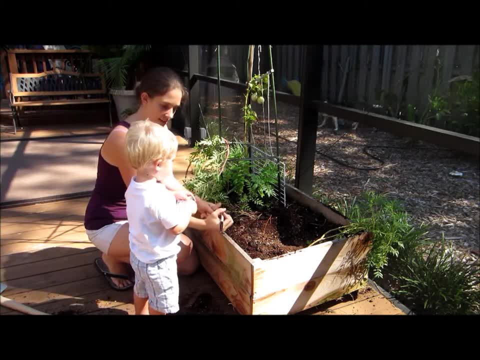 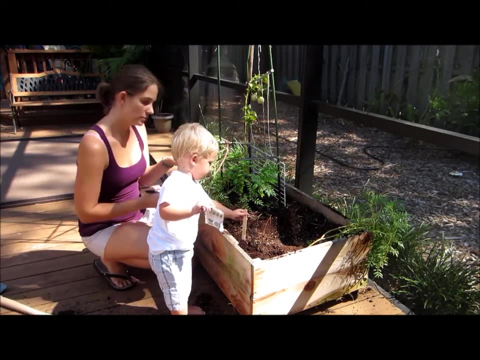 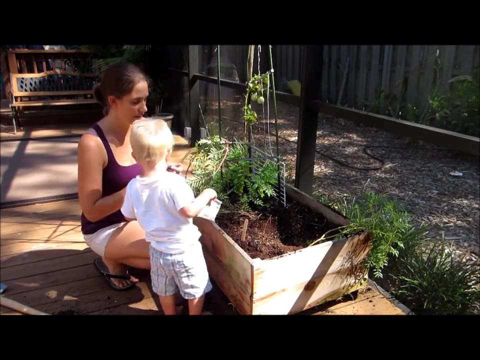 we need to write our word peas. Nicholas, you want to help me write? You want peas. Peas starts with peas. You want to help me write it? Oh, you want to just stick it. okay, Older kids can help write. since he's the only one, I'll write it for him. Okay, we need to stick. 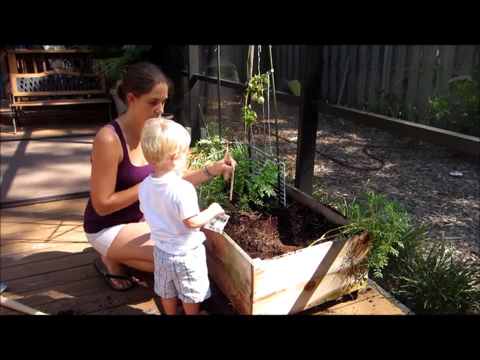 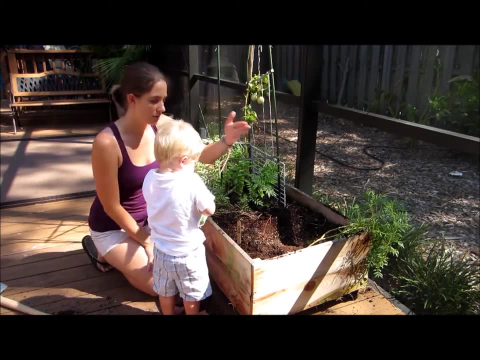 it in the dirt with the letters up: Okay, so grab it, push it in. Great job. that way we'll know that this is going to work Where our peas go. Now we're going to make a trench, and a trench is just like a V in. 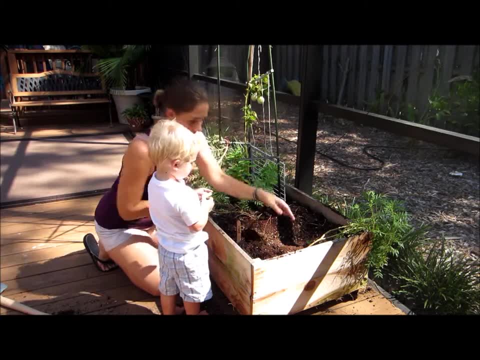 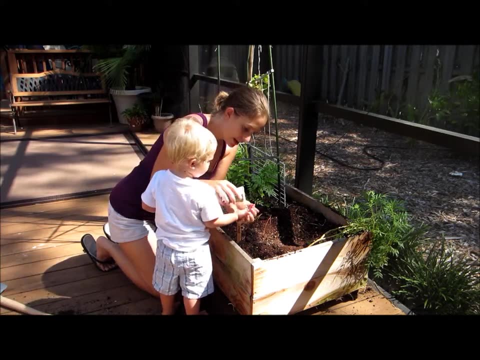 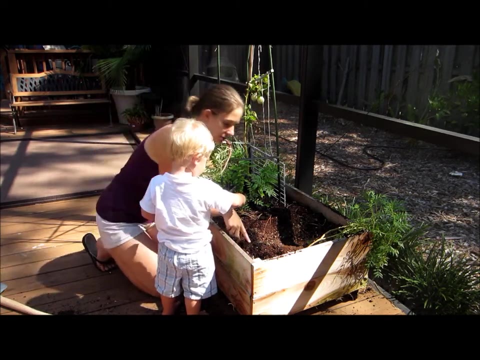 the ground In our dirt. Okay, Put your hand out flat just like this Ready, I'm going to put some peas in. We're going to take one at a time and put them in the dirt. That's right, One at a time. Put them separately. 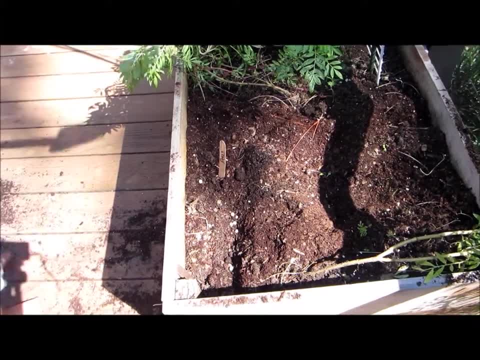 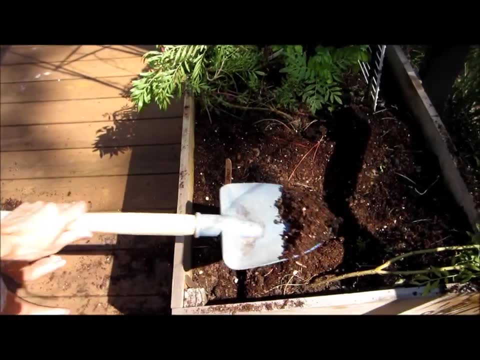 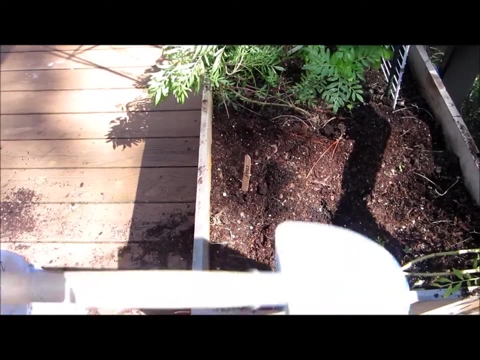 Okay, Nicholas, Now it's. You're right, we're going to need to cover it. We probably don't need a shovel to cover it. We could probably just cover it with our hands. That's a shovel? Okay, cover it up. Now let's cover it with our hands. Can you use your hands to cover it? Nope, you're. 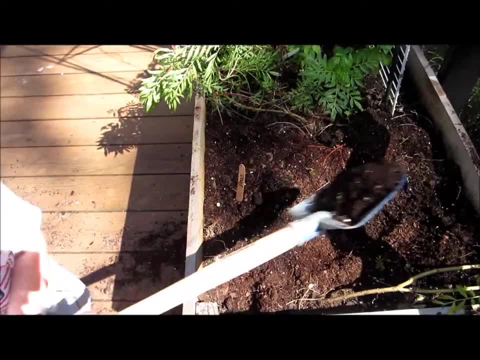 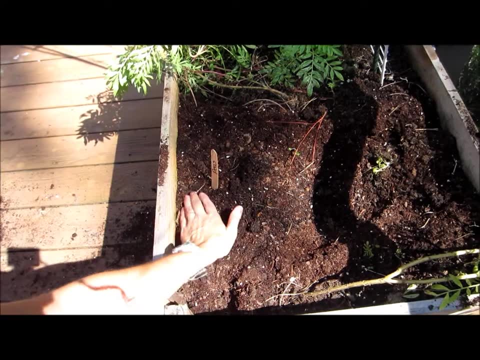 in the mood for a shovel? Okay, let's use your shovel to cover it. Now we're going to tuck them in. Nai Nai, Nai Nai. Okay, so take your hand and pat, pat, pat. Can you help me, pat?